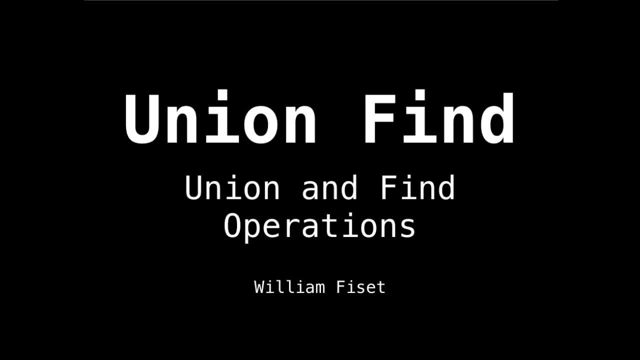 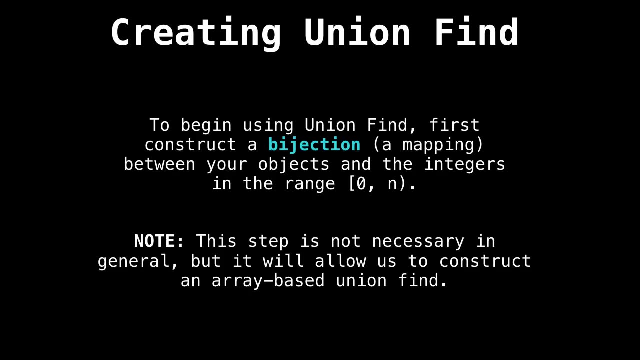 Okay. so now we're going to talk about the union and find operations we can do on the union find or the disjoint set. This is the video where I demystify how those actually work internally. So to create our union find, the first thing we're going to do is we're 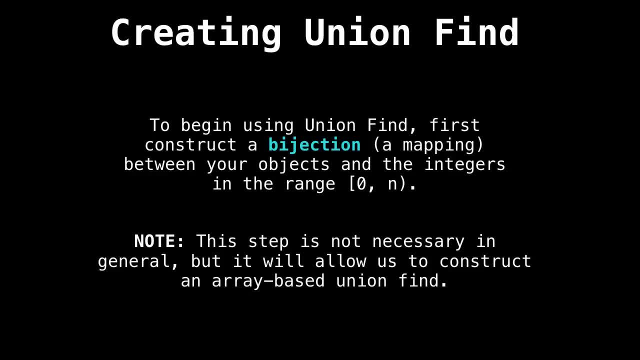 going to construct a bijection, or simply a mapping between our objects and the integers in the range zero inclusive, to n, non inclusive, assuming we have n elements. So this step in general is actually not necessary, but it's going to allow us to create an array. 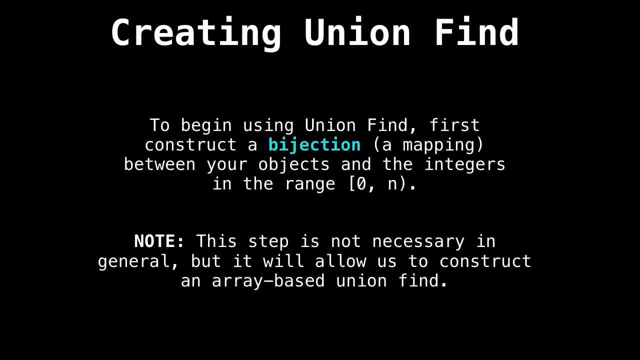 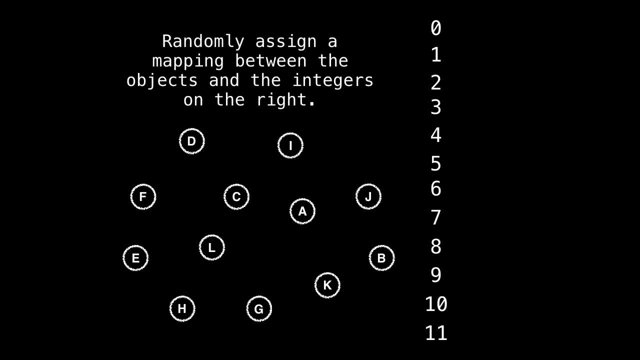 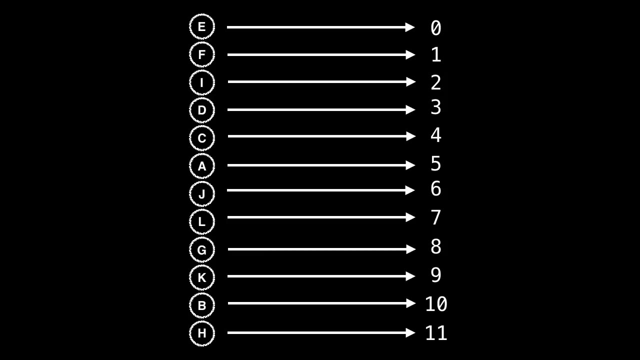 based unit find, which is very efficient and also very easy to work with. So if we have some random objects and we want to assign a mapping to them, then we can do so arbitrarily, As long as each element maps to exactly one number. So that is my random bijection And 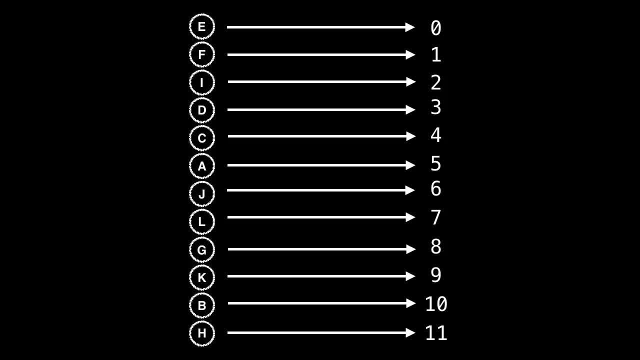 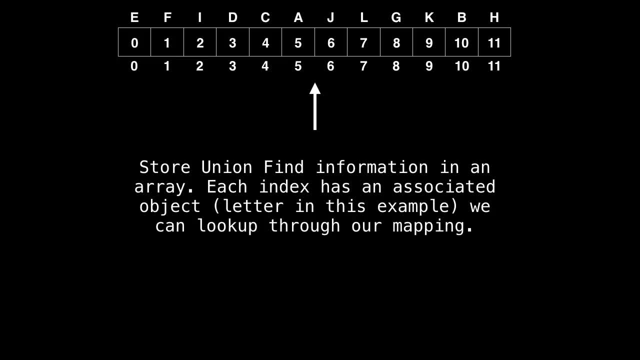 we want to store these mappings, perhaps in a hash table, so we can do a lookup on them and determine what everything is mapped to. Next, we're going to construct an array, And each index is going to have an array, And each index is going to have an array, And. 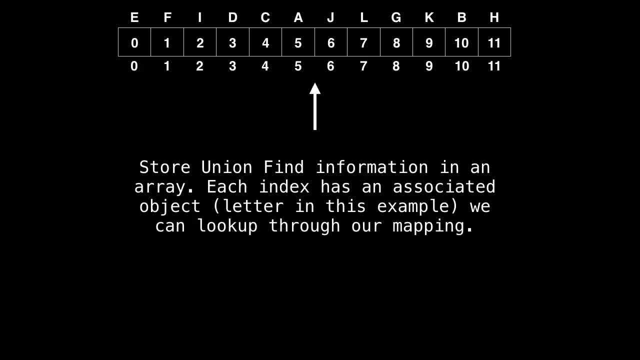 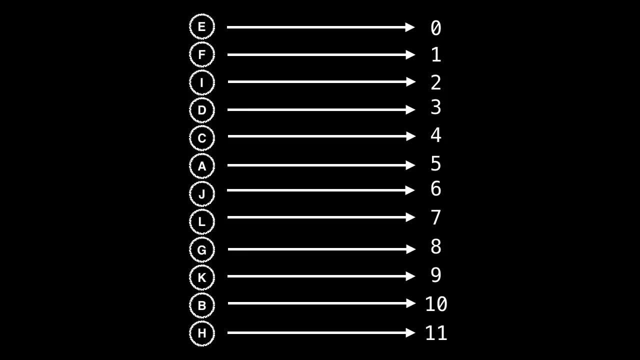 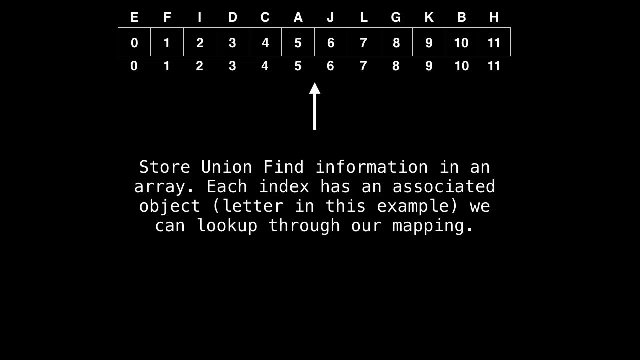 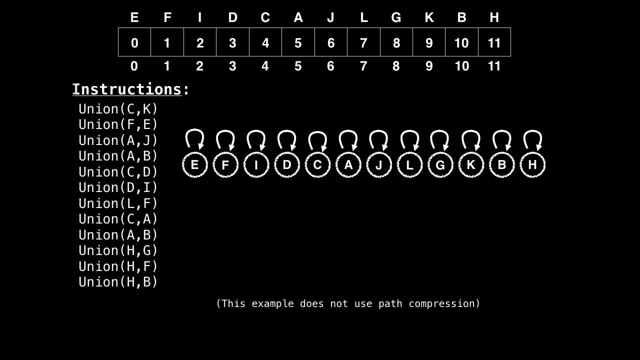 each index is going to have an array And an associated object and this is possible through our mapping. So, for instance, in the last slide, a was mapped to five, so slot five or index five is going to be a slot. So what you see in this picture is at the 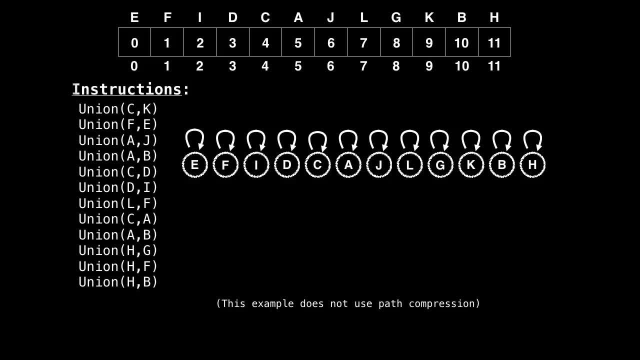 top is that array we just created which contains our mapping, And in the center is just a visual representation of what's going on. The value in the array for each position is currently the index which it is at. This is because originally every 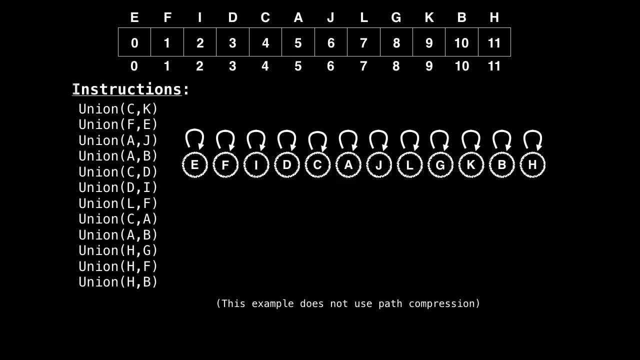 node is a root node, meaning it maps to itself. But as we perform the instructions on the left of unifying groups together or objects together into groups, we're going to find that we're going to change the values in our array to map to other letters. And specifically, 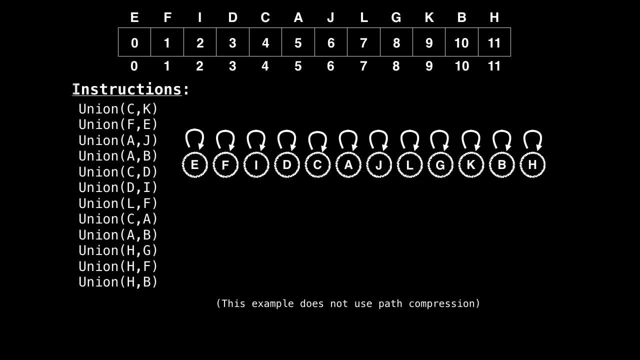 the way we're going to do it is for some index i in our array, index i is parent is going to be whatever index is at position i. So, for instance, if we want to unify c and k, we look at c and k. 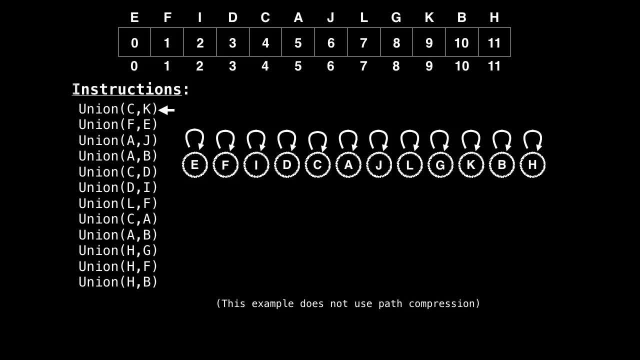 and we discover that c has a root node of 4 and k has a root node of 9.. So either c is going to become k's parent or k is going to become c's parent, And I chose that k's parent is going to be c. 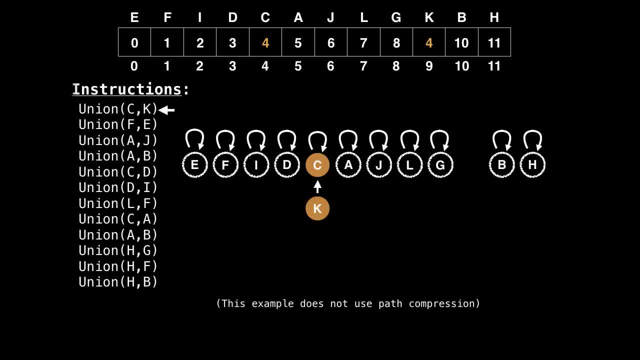 So now, at index 9,, which is k's position, I'm going to put a 4, because I know that c is a 4.. So next, f and e, we're going to do a similar type of thing and I'm going to say that. 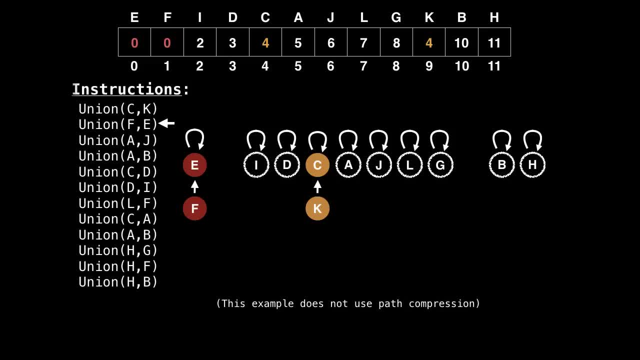 f's parent is going to be e. So at f's position, which is 1, I'm going to put a 0, because e is 0.. Similar thing for a and j. But here's where things get a bit more interesting. So now we want to unify. 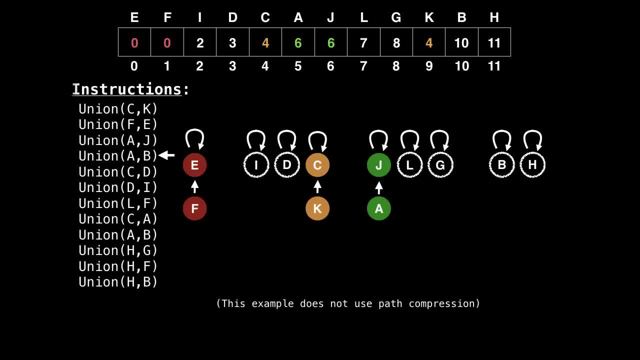 a and b. So if I look a, a has a 6 in its cell, but 6 is j. So I know that a's root node for group green is j And b is a single node because it's a self-loop. 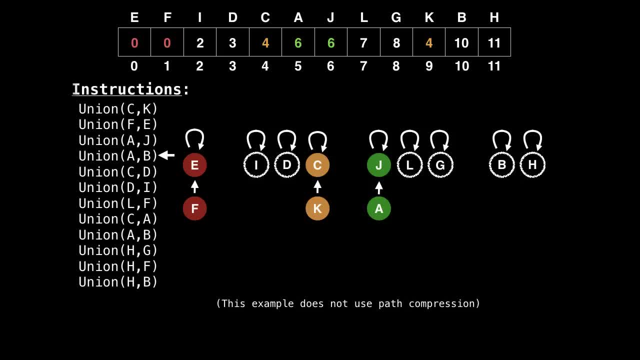 And in general I'm going to merge smaller components into the larger ones. So now b is going to point to j, because the green group's root node was j. So now we want to merge c and d. So I find the root node of 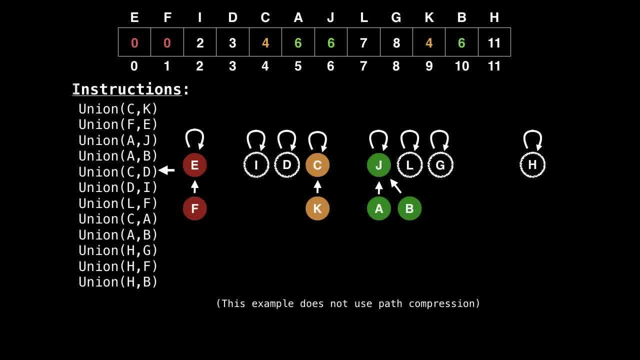 d, which is d, And find the root node of c, which is c, And I'm going to merge the smaller component, d, into the larger component, which is the orange group. So now d is going to be part of the orange group. 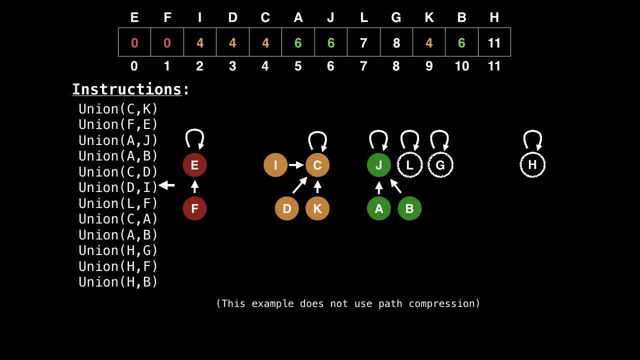 Now I want to merge d and i. So a similar thing happens and i now points to c. Now I want to merge l and f. So f's parent is e, So I'm going to merge l and to be into the red group. 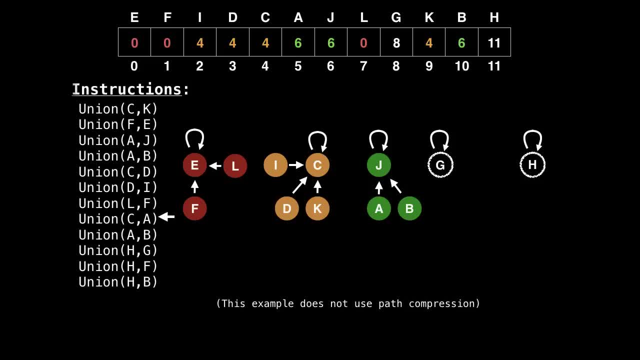 Now I want to merge c and a, So this is an interesting example. So I find c's root node, which happens to be c. I find a's root node, which is j. So now component orange has four elements, but component. 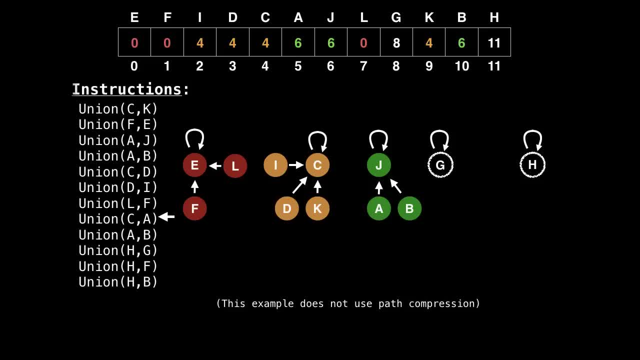 green only has three. So I'm going to merge the green component into the orange component. So now j is going to point to c, So I want to unify a and b. So if I go up and follow the parent nodes until I reach a root node, a's parent is j, j's parent is c. 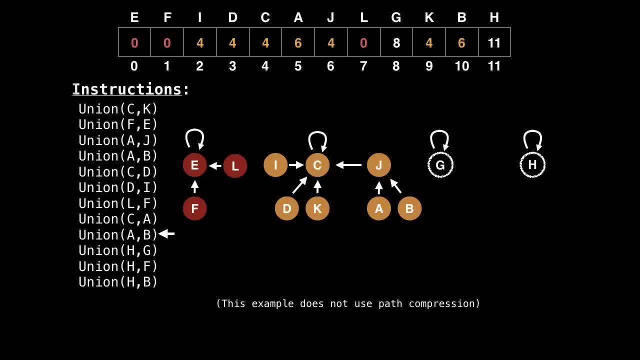 So I know that a belongs to the orange group, And if I do a similar thing with b, I also discover that b's parent is also c, which is the orange group. so I don't need to unify them, they're already unified together. so 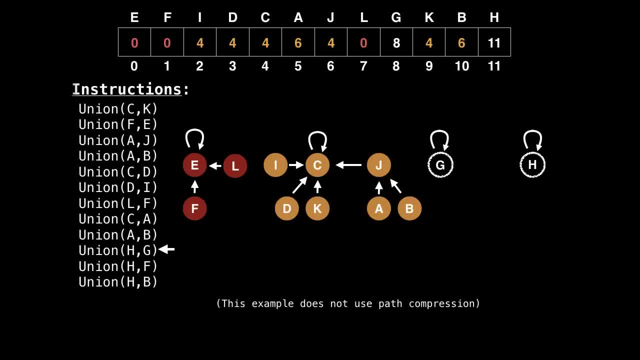 H and J G. they currently don't have a group, so I'm going to arbitrarily merge them into a new group, assuming to be the blue group. so H and F. so if I look, H is parent is G and F's parent is E, the right component is larger, so I'm going to 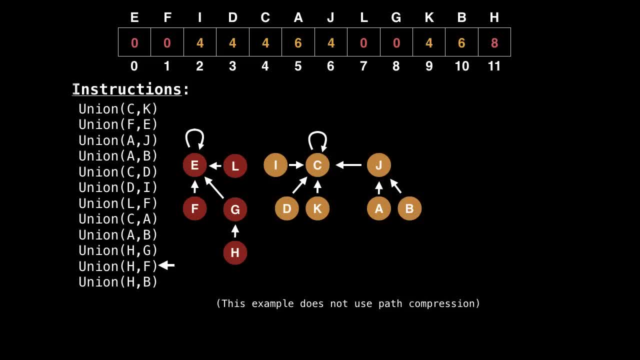 merge the blue group into it. and now, since G was the root node, I make it point to E, which was also the root node. now I want to merge H and B, so H's root node is E. if we follow up the chain from H to G to E, 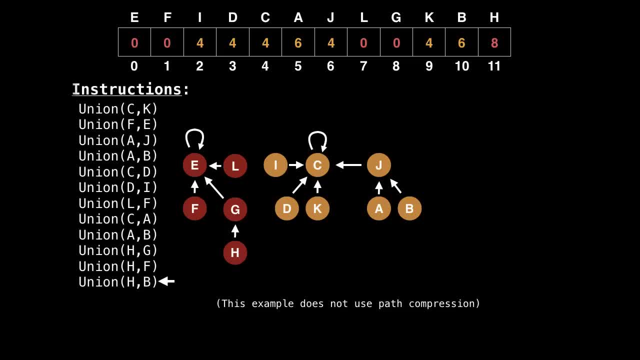 and B's root node is C, because we go from B to J to C. so now, since the orange component is larger than the red component, I'm going to point the root of the red component to the root of the orange component. so E now points to C. 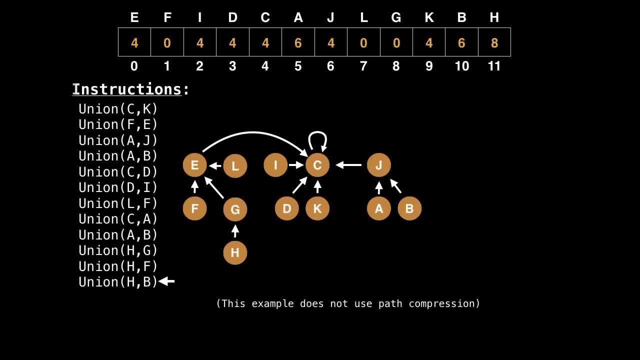 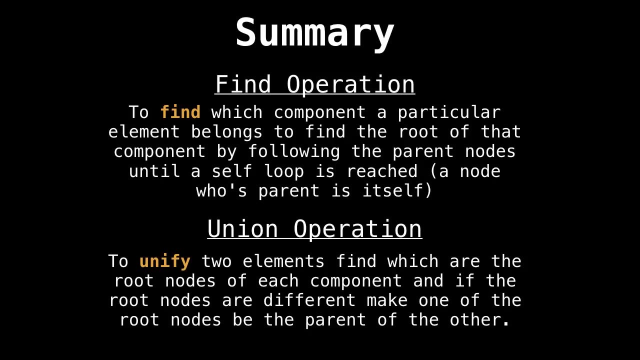 okay, and note that in this example, I'm not using a technique called path compression. this is something we're going to look at in the next video, which is an optimization on the union find. to summarize, if we want to find out which component a particular element maps to, what we have to do is find the root of that component by following all. 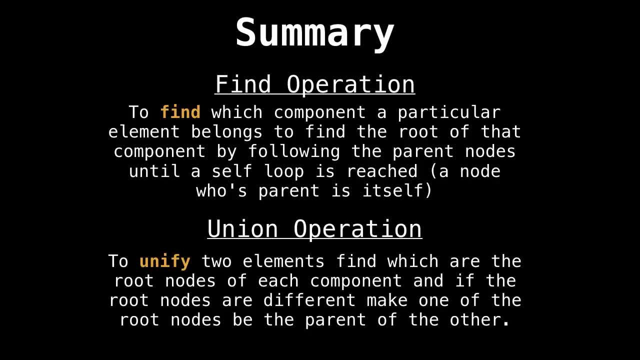 the parent nodes until we reach self loop or a node whose parent is itself, and that will uniquely determine which component that element belongs to. and to unify to the root of that component, we have to find the root of that component. so in this example we have two components together. what we do is we find the root. 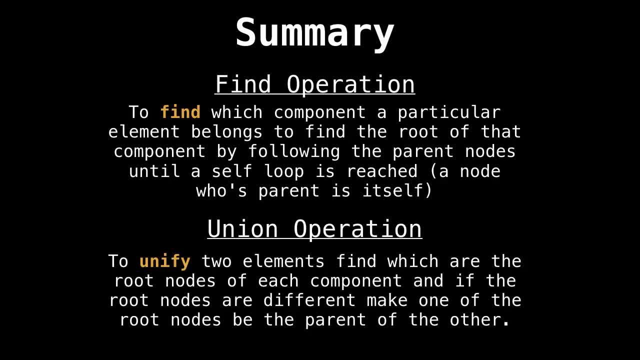 nodes of each component. and then if the root nodes are different- because if they're the same and then they belong to the same component already, so if they're different- make one of the root nodes point to the become the parent of the other root node. so just some remarks about this union. find data structure. so 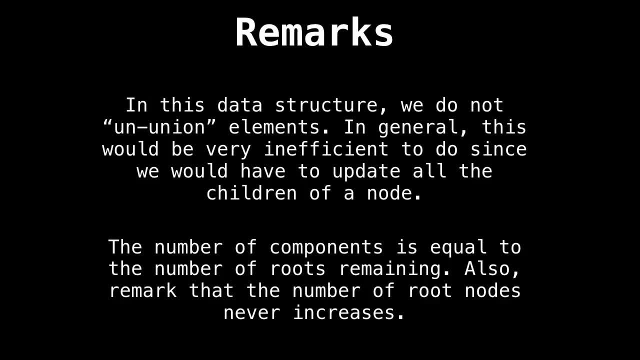 in general, we don't really need to use any treeえる just because this would be inefficient as we'd have to update all the children which point to that node and we don't have access to those. but we could probably, in theory, keep track of that. I just don't see any.